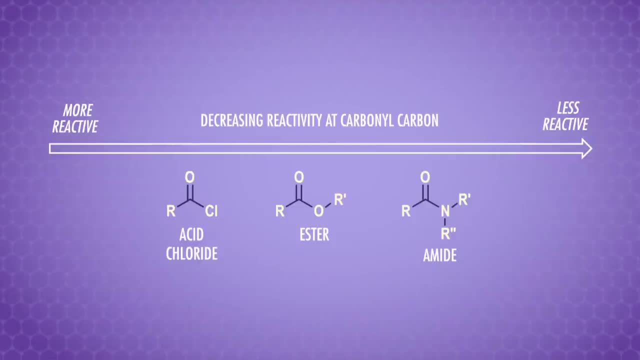 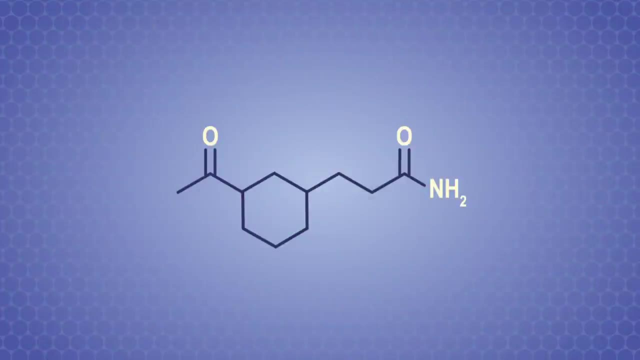 We looked at the reactivity of carboxylic acid derivatives in the previous episode. Let's add in the other carbonyl compounds we've encountered to give us the full picture. As an example, this molecule has two carbonyl functional groups: a ketone and an amide. 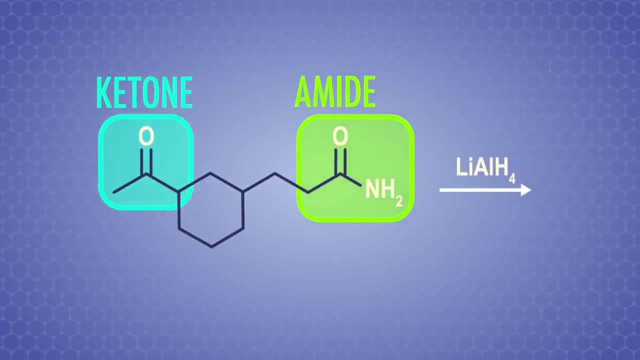 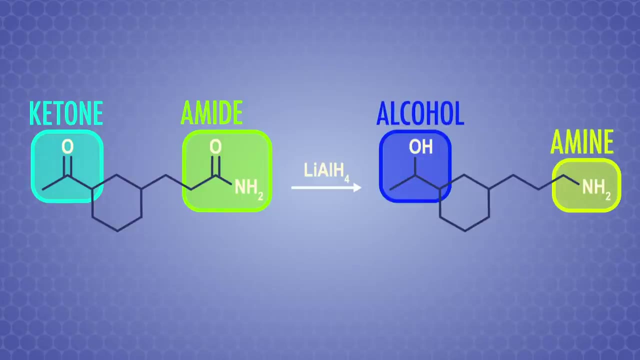 If we use a reducing agent like lithium aluminum hydride, that reactivity comes into play. The ketone gets reduced first into an alcohol and then the amide gets reduced into an amine. Lithium aluminum hydride is pretty much the sledgehammer option. 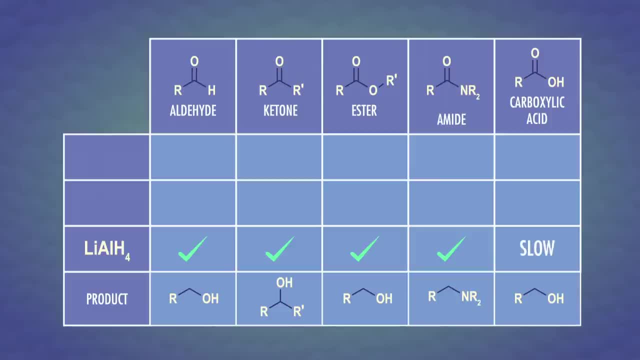 for reducing carbonyl compounds, as it can reduce them all. It can even reduce the less reactive carboxylic acids, albeit more slowly. If we want a bit more nuance, though, we can select a different reducing agent, like either lithium or sodium borohydride. 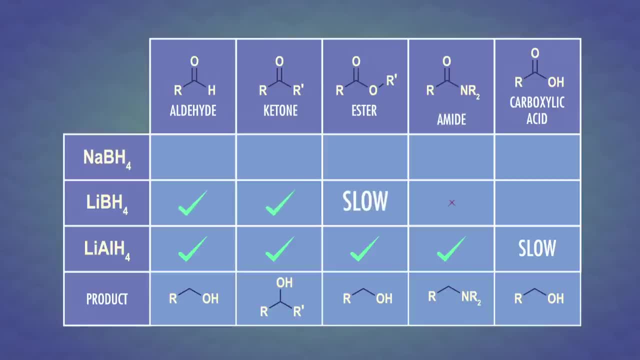 Lithium borohydrides can reduce aldehydes and ketones pretty quickly, or esters more slowly. Sodium borohydrides can reduce aldehydes and ketones, but it's speediest with aldehydes, Taking that molecule with two functional groups from before. 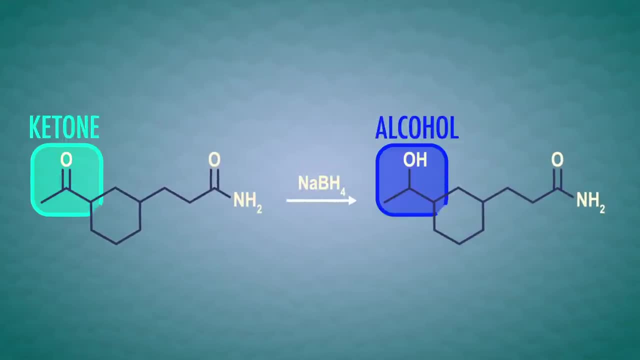 sodium borohydride can reduce aldehydes and ketones, but it's speediest with aldehydes. Sodium borohydride would be the perfect choice if we want to reduce the ketone but not the amide. But none of these reducing agents will help us reduce the amide but not the ketone. 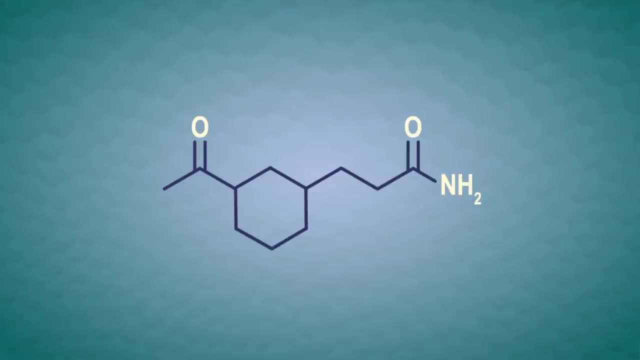 To stop the ketone from reacting, we need to cover it in our chemical painter's tape- a protecting group. Except because protecting groups can look really different depending on what they're covering or which reactant they're hiding from. it's more like giving the ketone a unique chemical disguise. 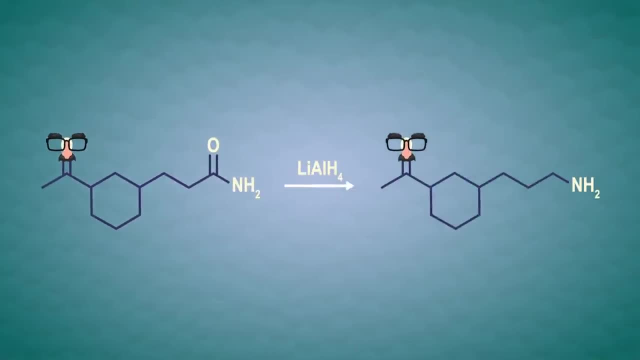 With some glasses and a fake mustache. our ketone is unrecognizable to lithium aluminum hydride And they don't react. The ketone can slip past the reducing agent undetected and take off the disguise once the reaction is complete. 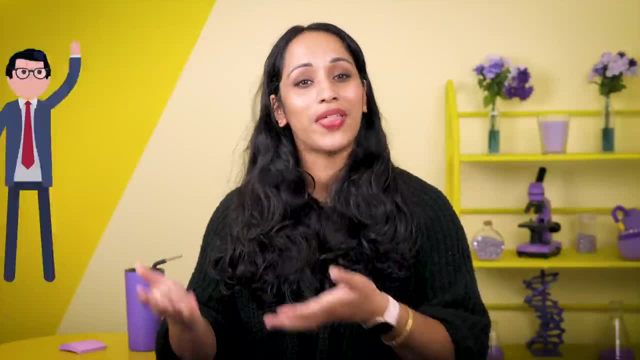 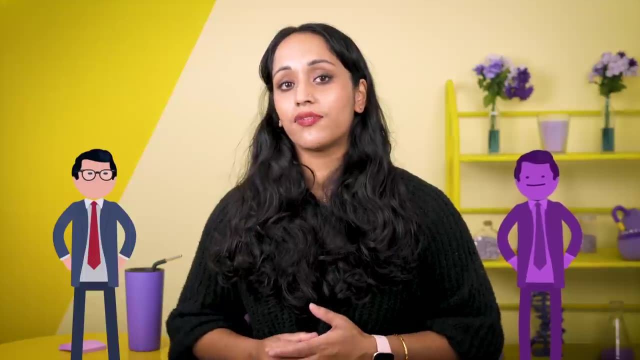 Mission accomplished. As we know from spy movies, there are both elegant and bad disguises, And the same applies for chemical disguises. There's a three-part checklist for a good protecting group One. it needs to be easy to attach to the part of the molecule we want to protect. We want to avoid multiple additional reactions or using inconvenient reaction conditions, Just like we want to smoothly change into a new spy outfit, not fumble around with an ironing board before swapping shirts. Two: it shouldn't react under the conditions we need to use later in the reaction. Because that might make it more difficult to remove afterwards. Just like we need a disguise to work in all locations, Traditional army camouflage is great in a forest, but not so great if we have to swim in the ocean too, Then our clothes are heavy and damp and a pain to change out of. 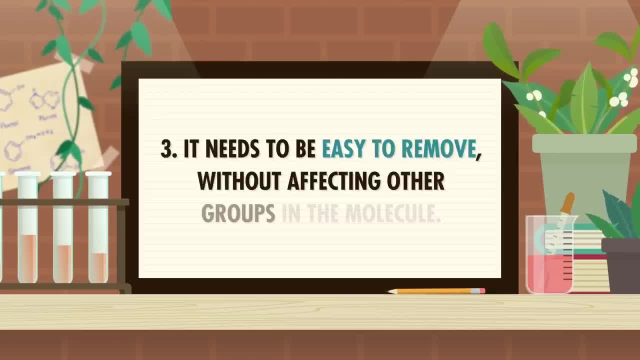 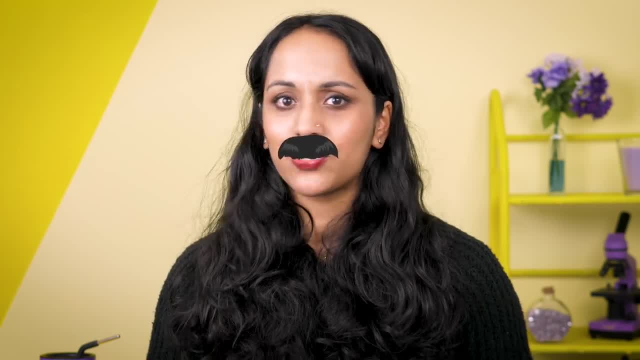 Three: it needs to be easy to remove Without affecting other groups in the molecule. If removing it requires a reaction that will change other functional groups in the molecule, we'll get a headache trying to change them back, Just like we want our fake mustache to come off easily. 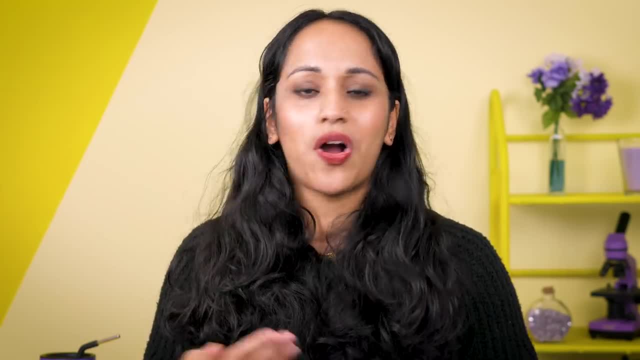 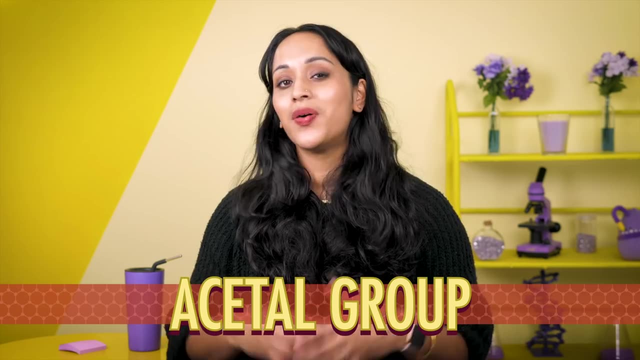 and without leaving incriminating glue marks or synthetic hair all over our clothes. For example, one way to protect aldehydes in ketones is to turn them into an acetal group. We met the acetal group in episode 29, when we added methanol to a ketone. 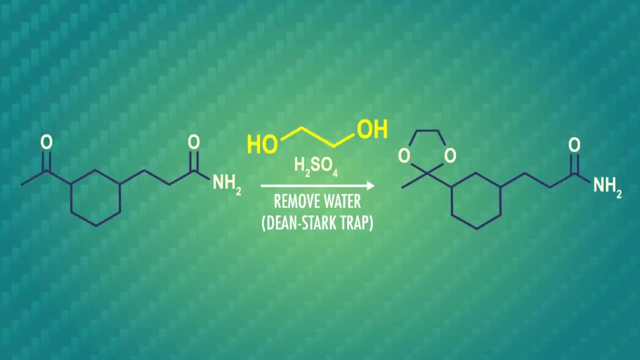 This group protects aldehydes in ketones from reactions with nucleophiles and bases, And the dial makes a cool little ring structure. With our protecting group in place, we can go ahead and react our amide with lithium aluminum hydride to convert it to an amine. 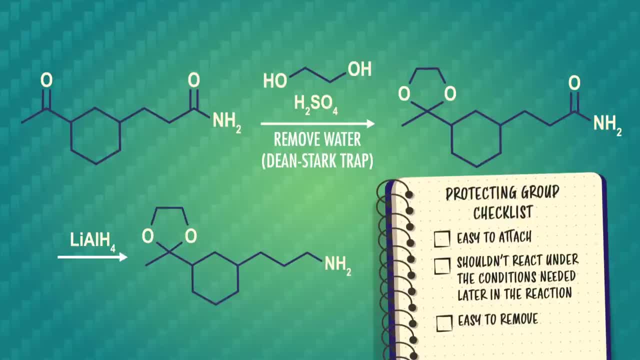 So far, so good. Our protecting group was easy to put in place, so that's one checkmark. And it hasn't reacted under the reaction conditions used to reduce our amide, so that's another check. All we need to do is add acid to hydrolyze our chemical disguise away. 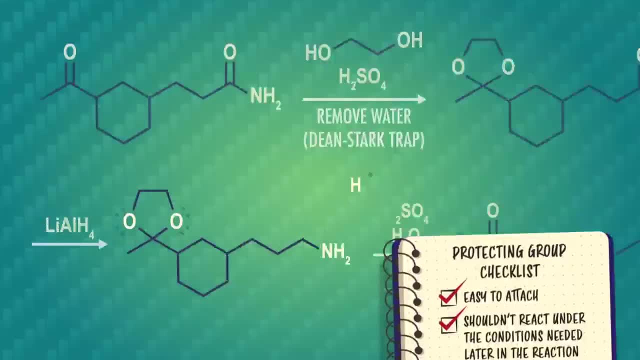 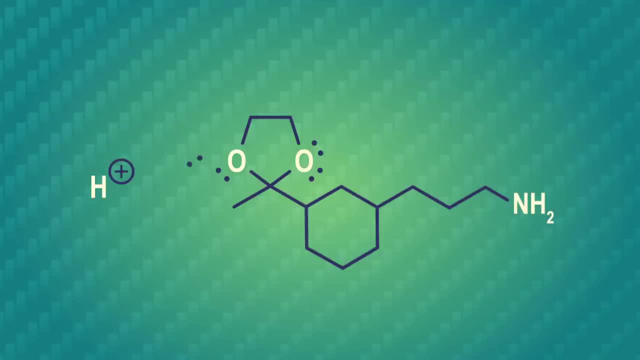 so it checks the final box of being easy to remove too. Let's take a closer look at this removal mechanism. One of the oxygens in the acetal group grabs a proton, which leads to one of the oxygen-carbon bonds breaking with a push from the neighboring oxygen. 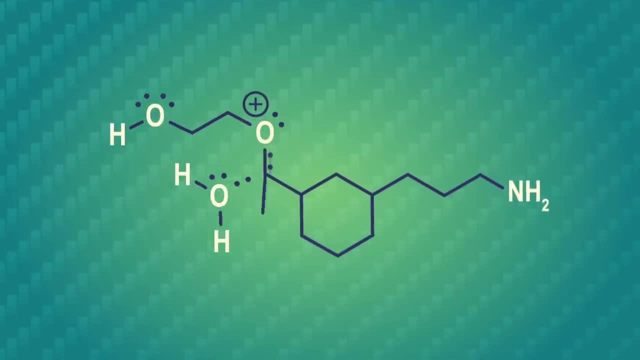 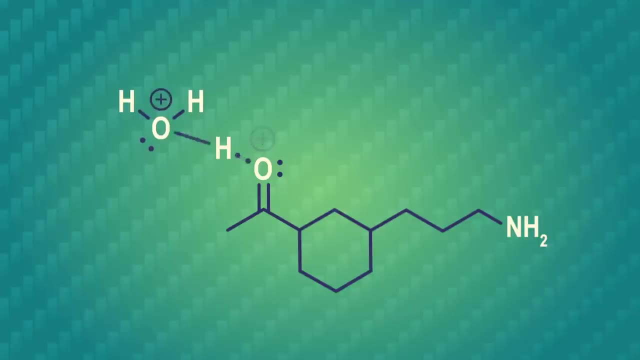 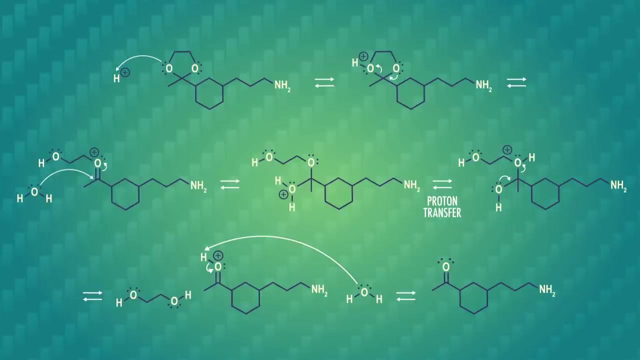 Next a water molecule swoops in, kicking off a chain of proton transfers and electron movement which eventually forms an oxonium ion. Then a final water molecule plucks the hydrogen off of the oxonium to remake the ketone. So with help from an acetal-protecting group, we can reduce a carbonyl group. 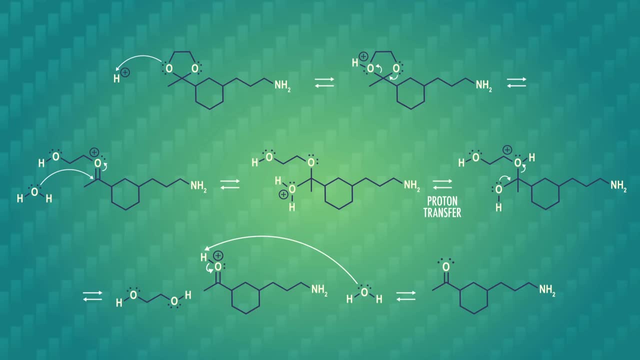 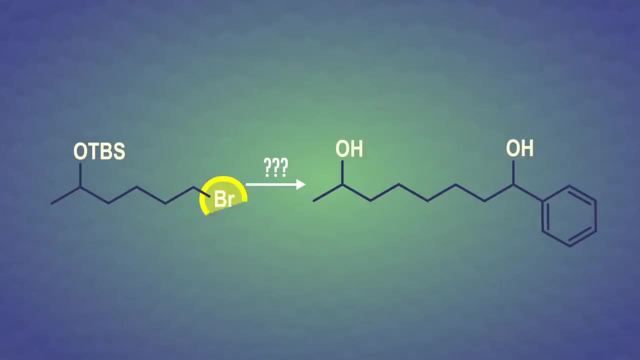 even if it's less reactive than other carbonyl groups in the molecule. We don't just use chemical disguises with carbonyls, though. Take a look at this reaction. We want to remove the bromo-functional group on the right-hand side of the starting material. 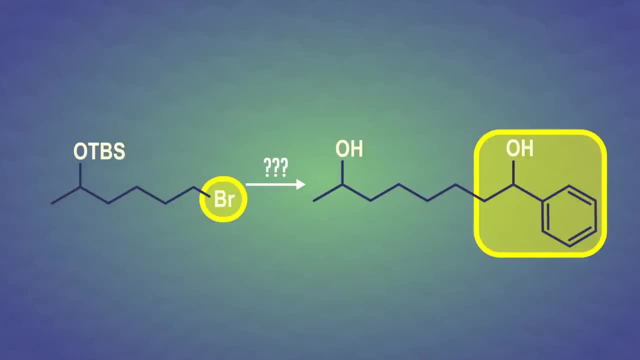 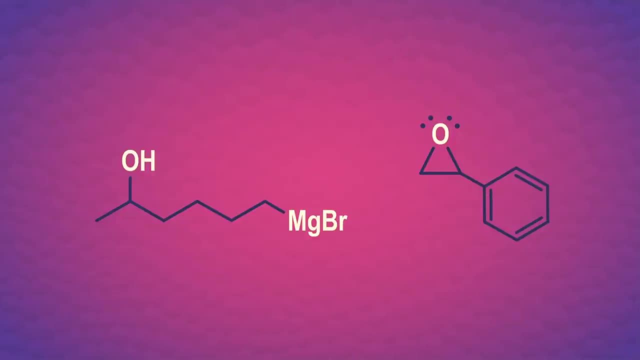 and replace it with an additional alcohol and phenyl group. Let's start by comparing the number of carbons in our starting material and product to see where we need to form a bond If we can transform our starting reagent into a grignard. 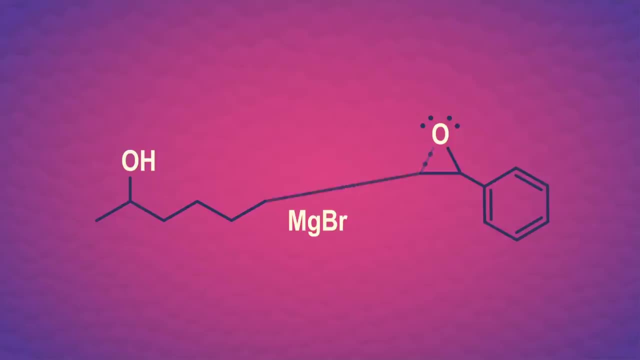 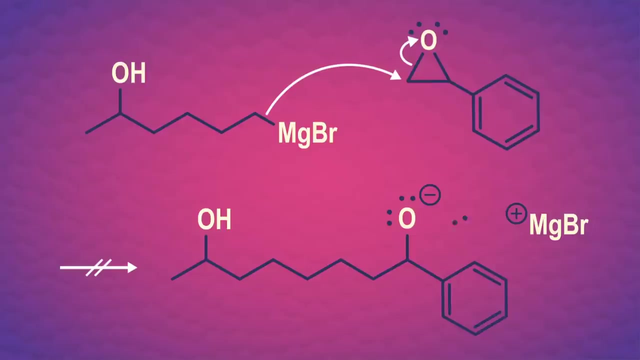 we could hypothetically use it to join onto an epoxide, like we learned in episode 24.. But wait, There's a problem. Grignards will react with alcohols in an acid-base reaction. So as soon as we form the grignard, we won't get the reaction we want. 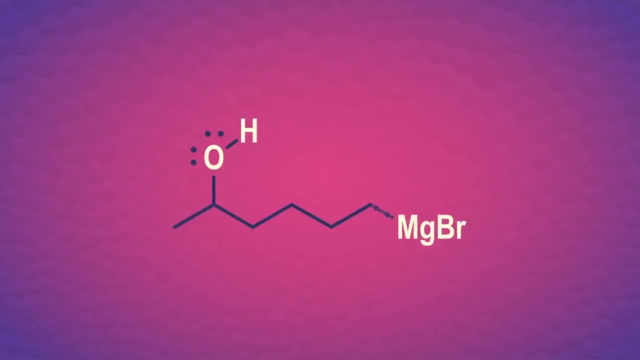 Our grignard molecule could react with itself, deprotonating the alcohol group on the other end, or it could react with another reactant molecule. Either way, we're nowhere near the product we wanted to make, So we'll need a protecting group. 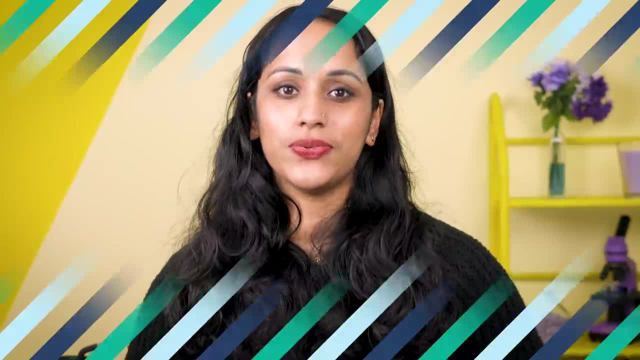 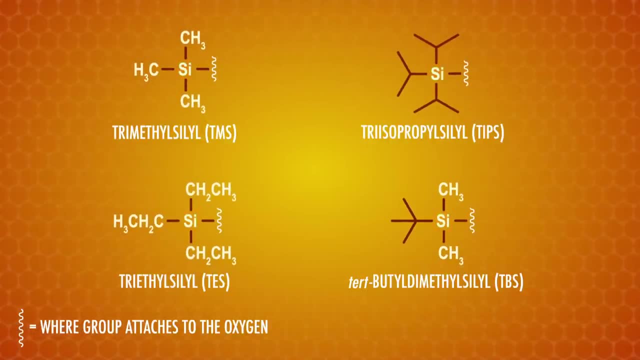 And there are two classic chemical disguises that alcohols can use. One option is siloethers with a silicon atom covalently bonded to an alkoxy group. There are a few different varieties with different alkyl groups attached. 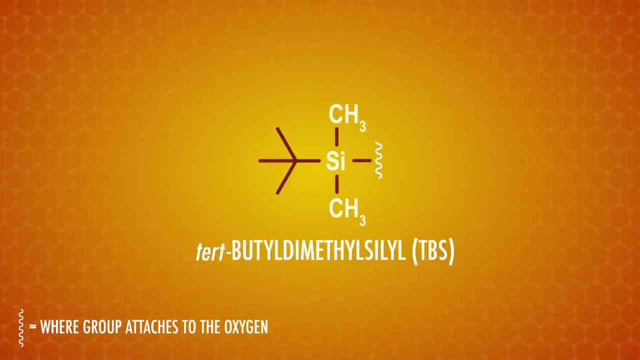 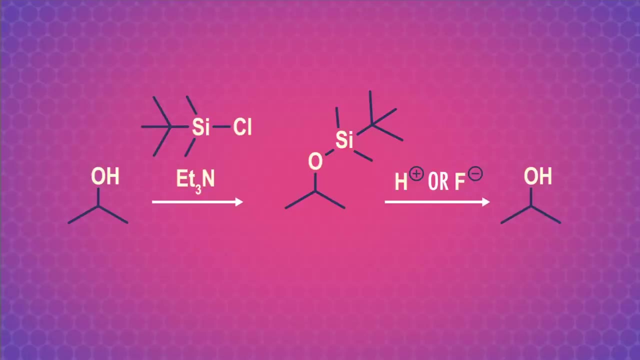 but the one we'll use here is tert-butyl-dimethyl-siloether, or TBS for short. So let's react our alcohol with TBS, chloride and triethylamine, which will snag the hydrogen. that's on the OH group. 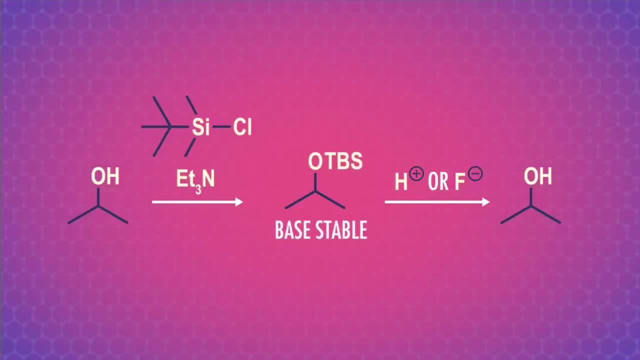 The newly attached TBS protecting group can't be removed by a base and we can remove it later by reaction with fluoride. Smaller siloel groups come off easily in acid, but the chunky siloethers are a little more resistant and more commonly used in practice. 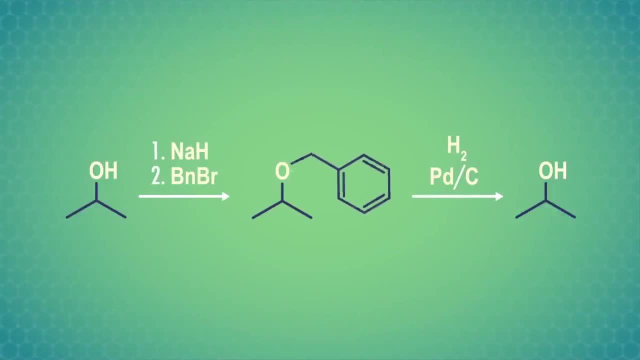 A second protecting group option for alcohols is a benzyl group- BN for short. We have lots of aliases for our disguised molecules which help us from having to draw out big protecting groups in our reaction mechanisms. We can attach this protecting group by reacting the alcohol. 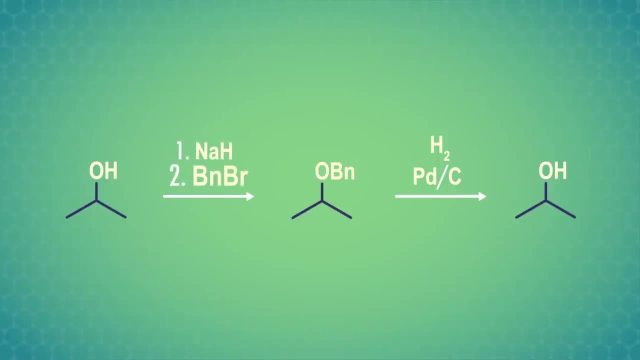 with a strong base, like sodium hydride and a benzyl halide. The benzyl group has an advantage over the siloethers because it's not removed by bases and it's also tricky to remove in acidic conditions. However, it has to be removed by hydrogenation. 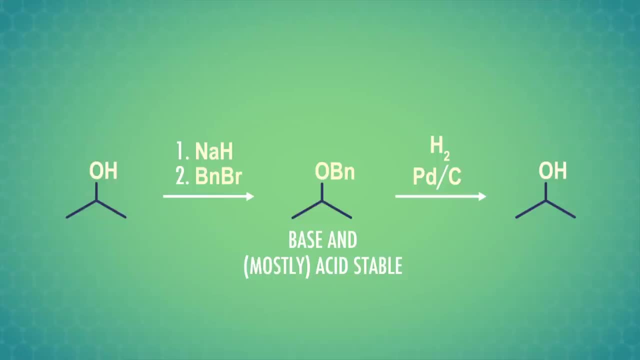 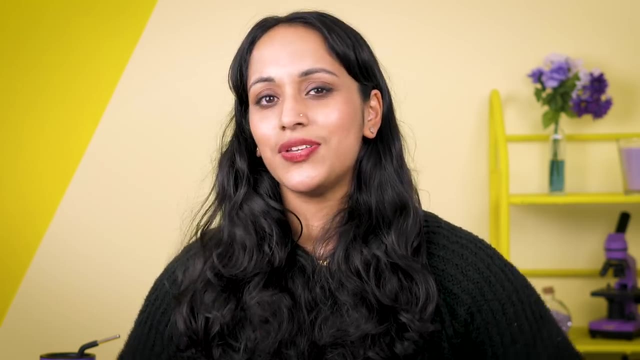 which might be a problem if you have double or triple bonds in your molecule. For the Grignard-related reaction puzzle we were looking at, either of these alcohol-protecting groups will do, but let's just use a siloether Before we form a Grignard or anything though. 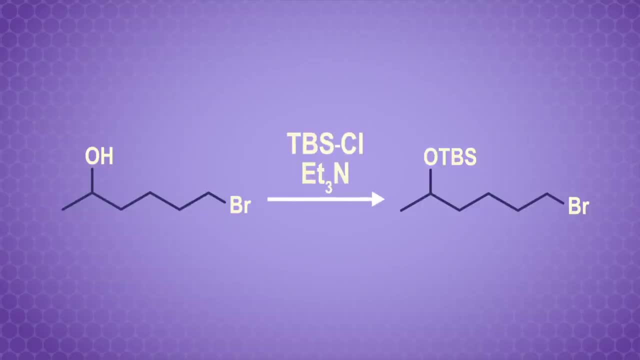 we need to add a protecting group using TBS, chloride and triethylamine as our base. again, TBS takes the place of the hydrogen on the alcohol group and our chemical disguise was easy to add. so that's one of the three checks on our good protecting group checklist. 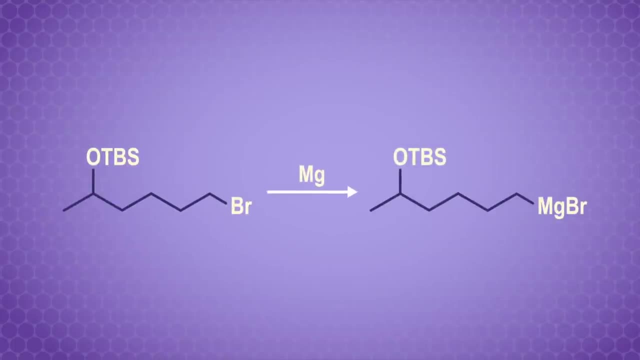 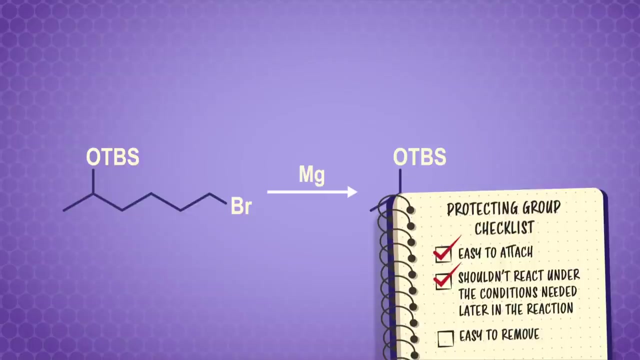 Now we can form a Grignard by reacting with magnesium. Our protecting group is disguising the alcohol, preventing those acid-base reactions we don't want, So not reacting under the conditions of the reaction Check. This means we can go ahead and form the product we want by reacting with this epoxide. 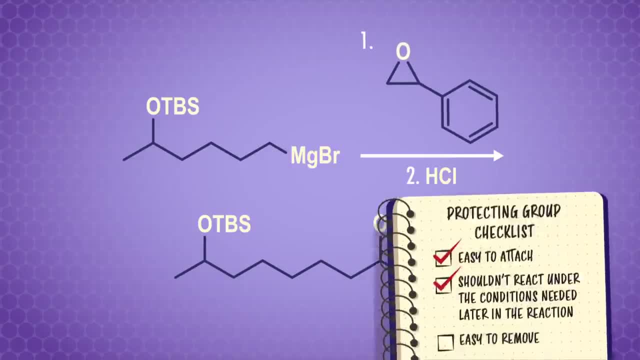 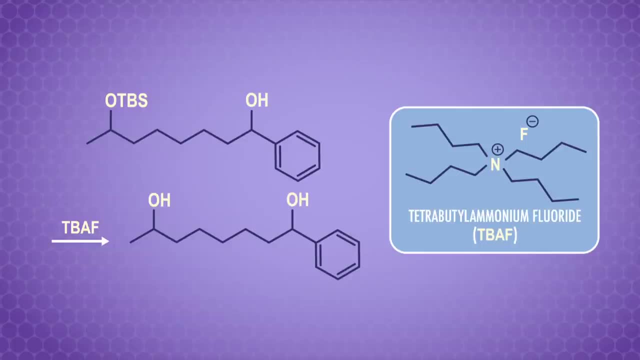 Again, the protecting group remains unchanged during this reaction. so double check to that second box. Finally, it's time to remove the protecting group with an acid or a fluoride, In this case tetrabutyl ammonium fluoride, or TBAF for short. 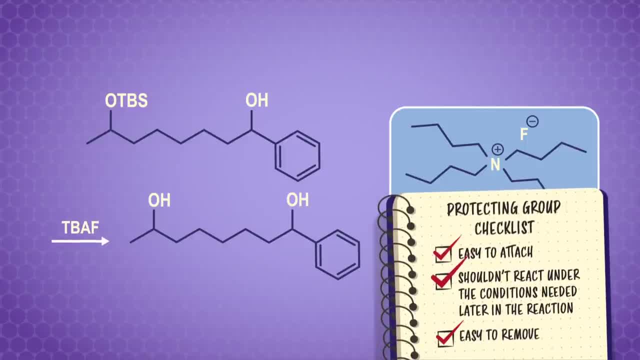 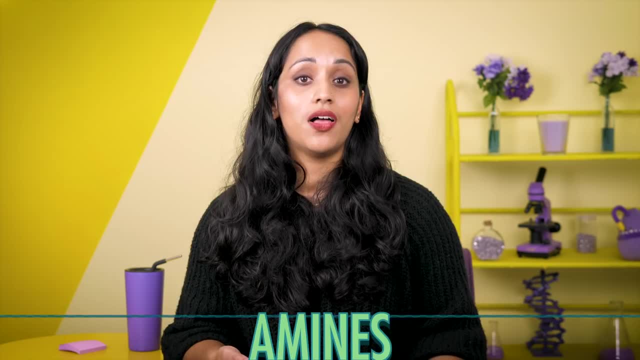 Our alcohol protecting group is easy to remove Check. Just in case you had doubts. there's the checklist proof that siloethers are good chemical disguises. In addition to carbonyls and alcohols, amines are another common secret agent. 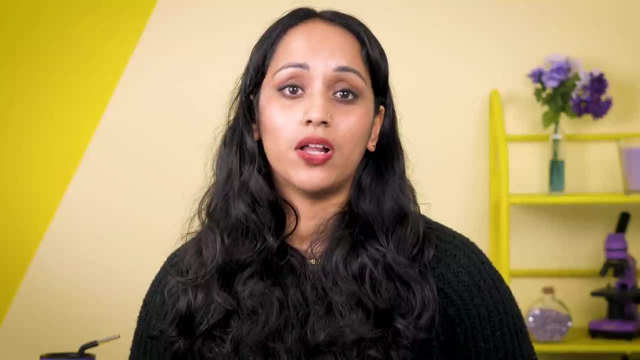 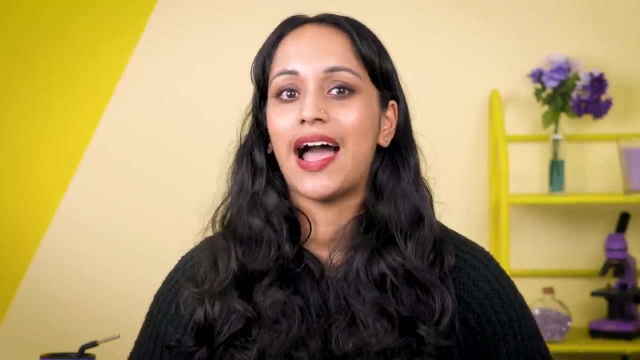 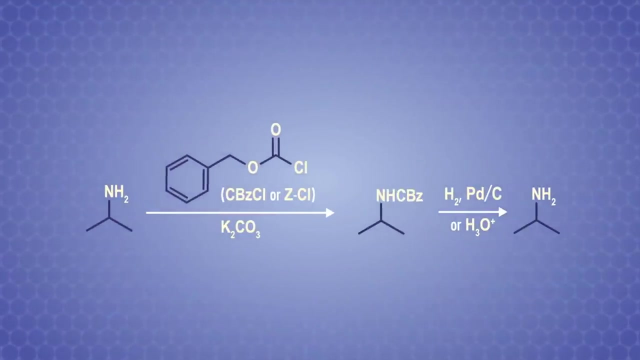 Well, functional group Amines pop up often in organic molecules and their nucleophilic and basic nature means that they can easily get involved in unwanted reactions if we don't disguise them. And we have three main choices. One option is adding a carboxybenzyl group, CBZ, or Z for short. 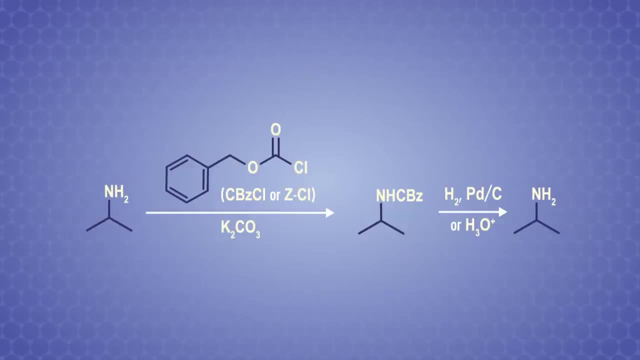 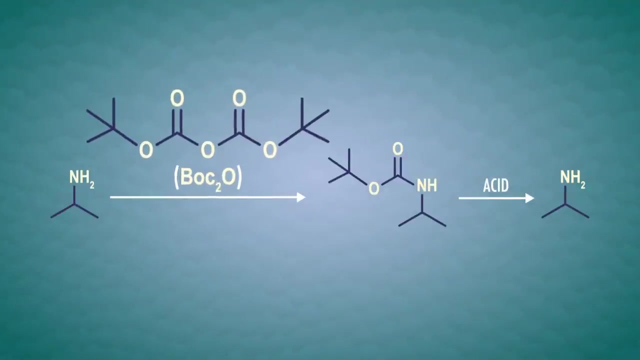 by reacting our amine with benzyl chloroformate. Later, we can remove this protecting group by hydrogenation or using a strong acid. A second option is diterbutyl dicarbonate, more commonly known as BAC anhydride. 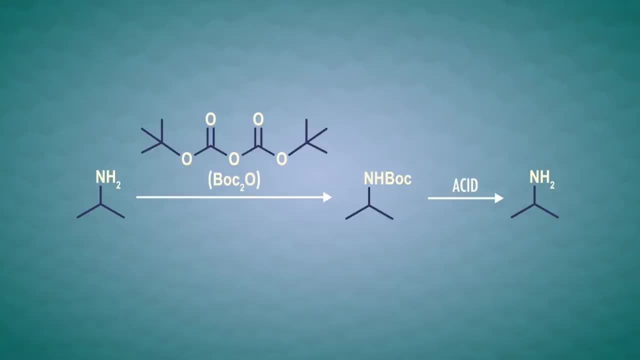 In the presence of a base, we add a tert-butoxycarbonyl or BAC group in one of the hydrogens on the nitrogen in the amine And we can remove it easily by adding acid. We can look to our model. 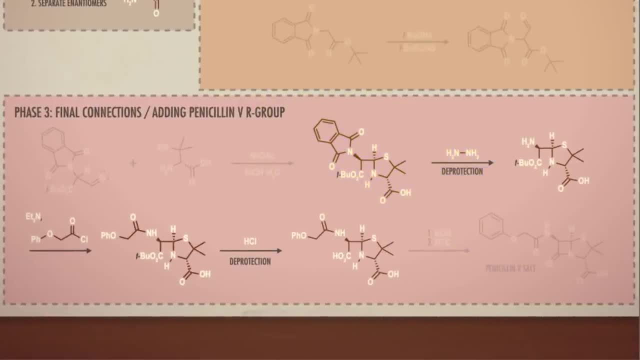 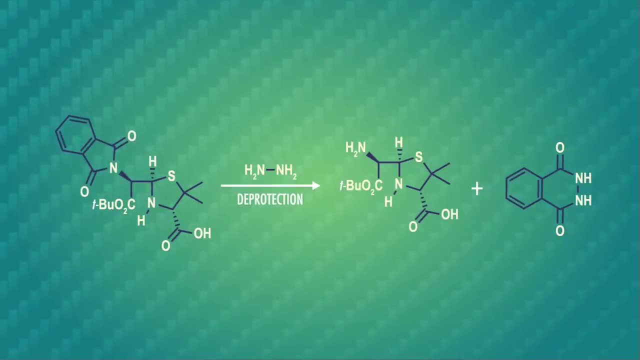 our mold medicine map and the synthesis of penicillin V. for our third and final amine-protecting group, ethylamide. This protecting group prevents the amine from reacting with an aldehyde in an earlier step of the synthesis. 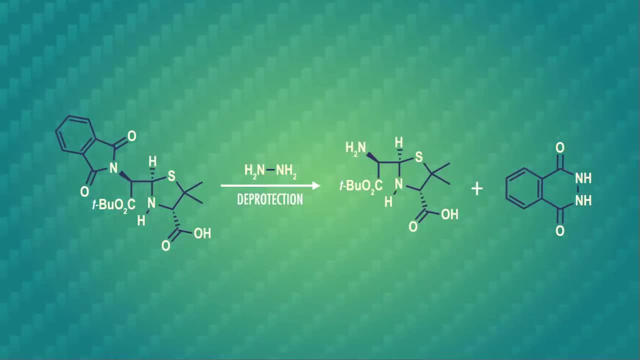 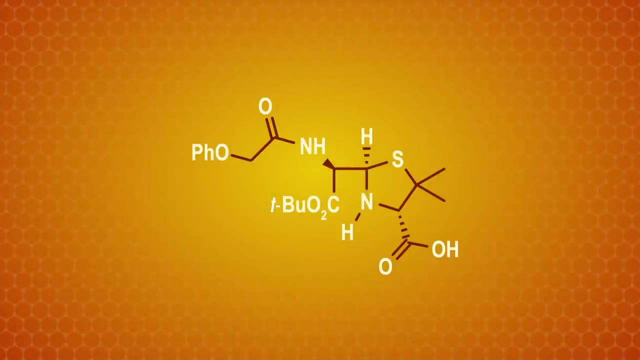 In this step it's being removed from our protopenicillin structure. The removal includes swapping the amide-like linkages to make a sort of double-amide side product. Plus, there's a bonus disguise in our mold medicine map: We can protect carboxylic acids by bulking them up. 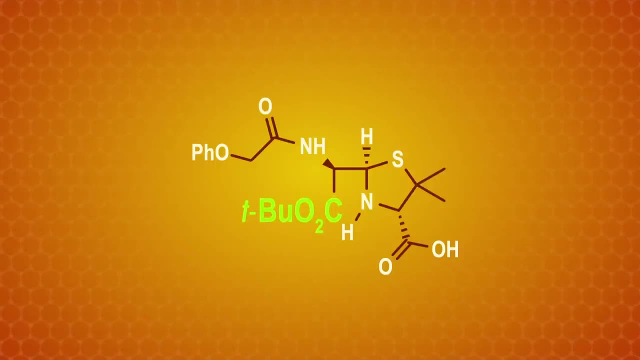 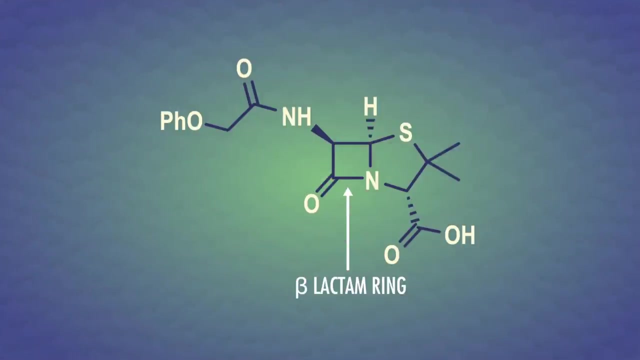 pumping out the hydrogen on the OH group to form a tert-butyl ester instead, And this protecting group can be removed later with acid. Sheehan actually did this deprotection right at the end of the penicillin synthesis before making the strained four-membered beta-lactam ring.